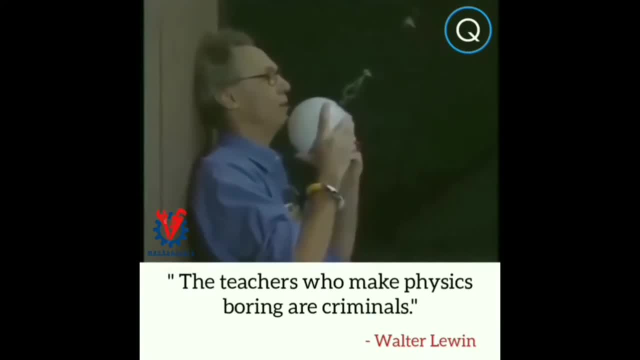 that when it comes back, it may touch my chin, but it may not crush my chin. I want you to be extremely quiet, because this is no joke. I want you to be extremely quiet because this is no joke. If I don't succeed in giving it zero speed, then this will be my last lecture. 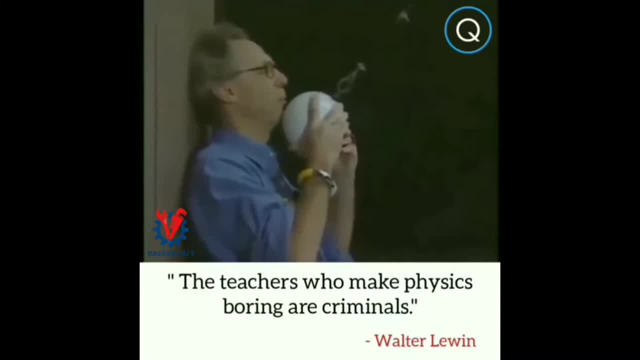 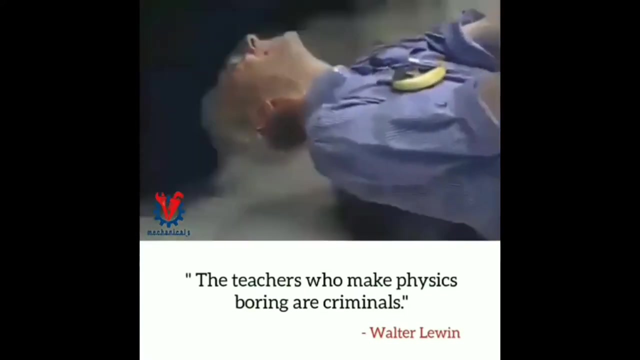 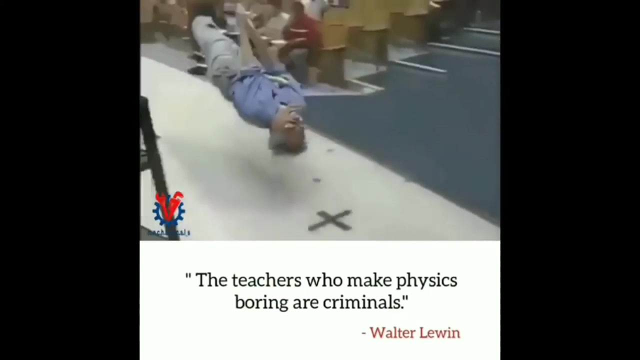 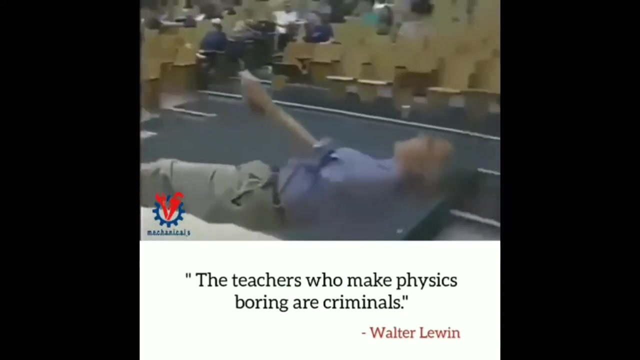 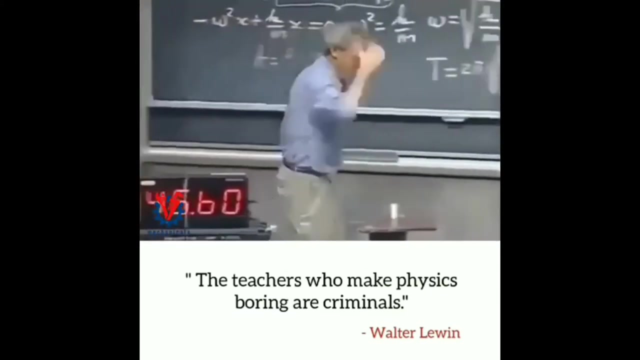 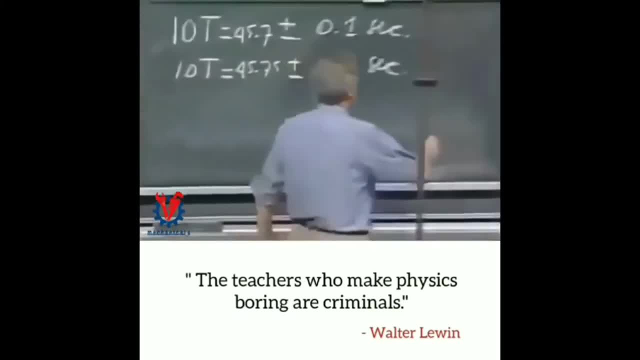 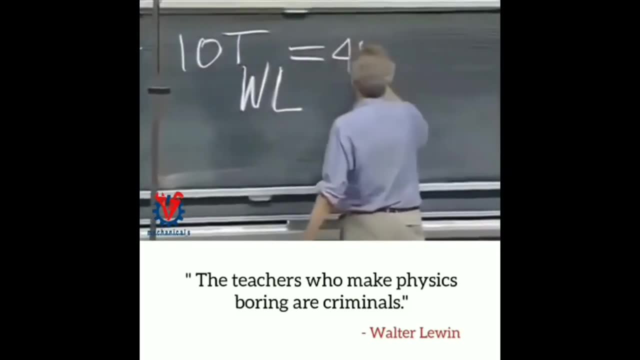 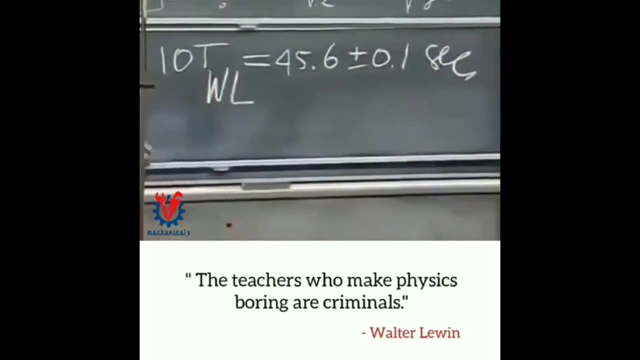 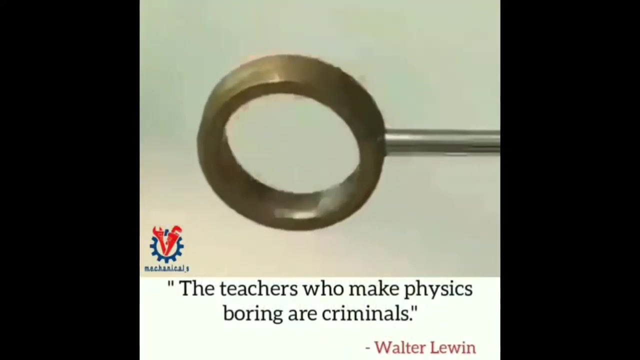 With Walter Lewin: 45.6.. Plus or minus 0.1 seconds. Physics works. I'm telling you. I'll see you Monday. Have a good weekend. This is the ring, And here is that brass ball Goes through there quite easily. 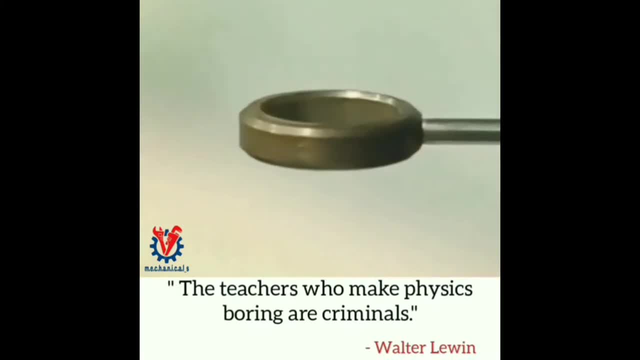 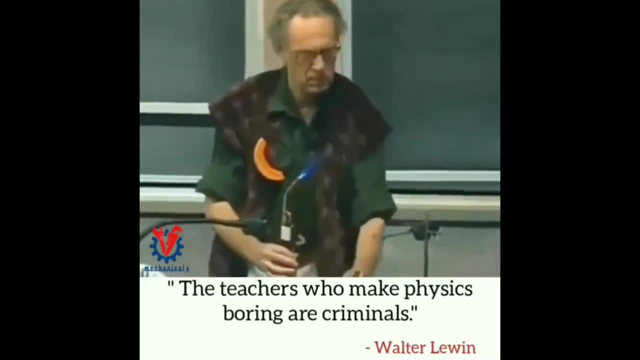 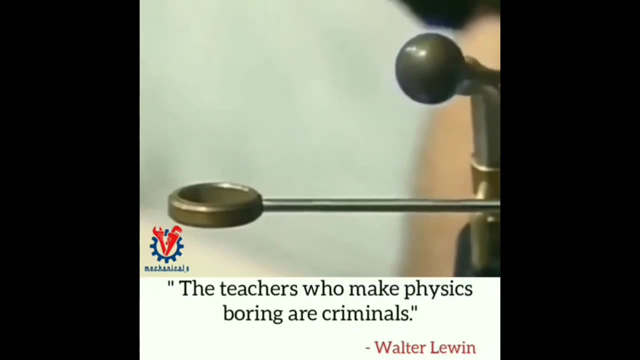 So I'll put it horizontal now, And then I will start heating up this ball. It's a ball. It can't be too close to the ring, because then the ring will also be heated, And then, of course, if the two have the same. 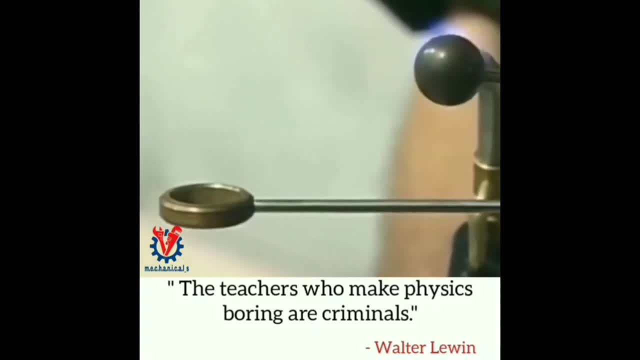 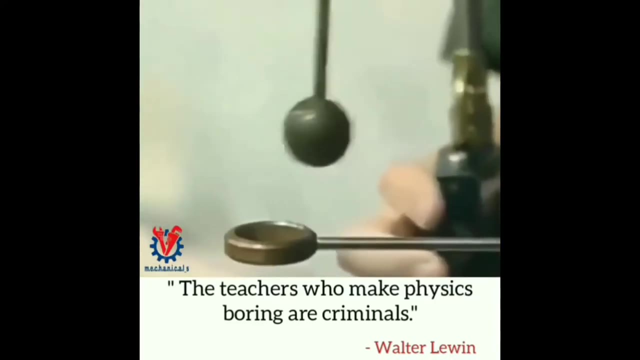 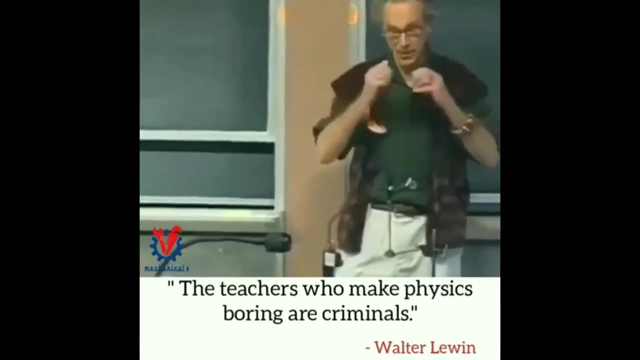 temperature, then the ball will still go through. Let's see Now. it doesn't want to go through, So we'll leave it like that and we'll see what happens. So the ring will now expand a little because it gets hotter and the ball will shrink a. 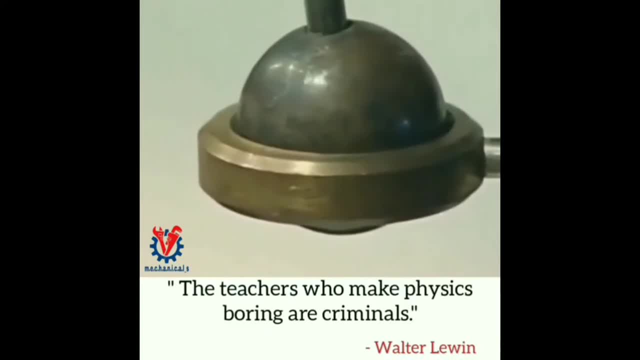 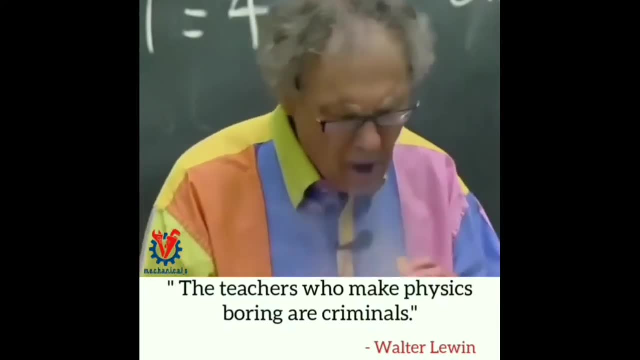 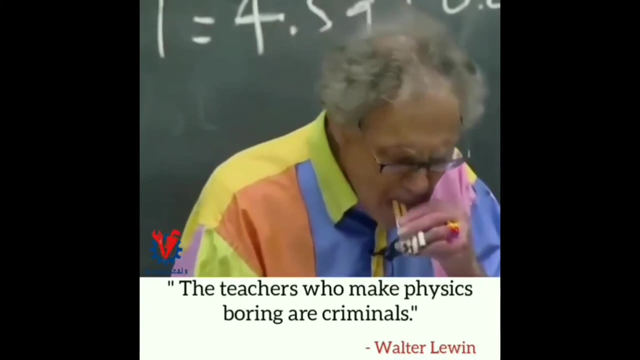 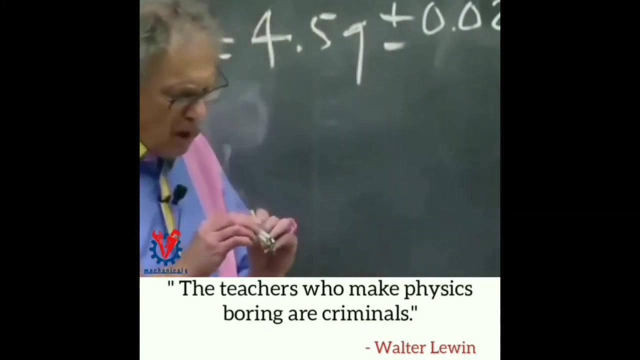 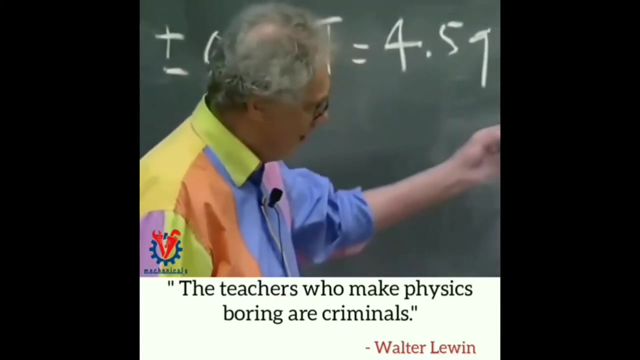 little, because it gets colder and it shouldn't take too long For the ball to be able to get through. OK, I'm going to make it completely dark and then I'm going to hold it in there. All lights off, All off. 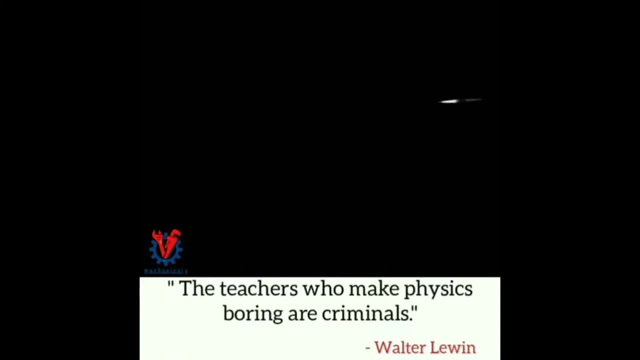 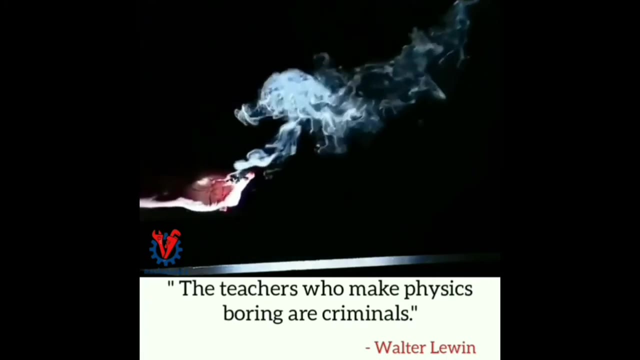 All off. So we all agree that this is white light which is coming up, and you don't see the light here because there is nothing that scatters it in your direction, So you don't see light here. But now look, Those of you who see blue say yeah. 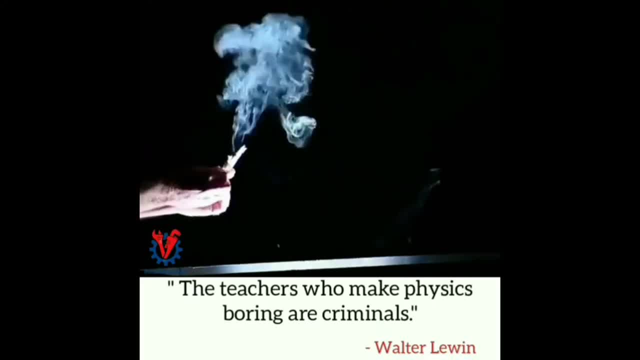 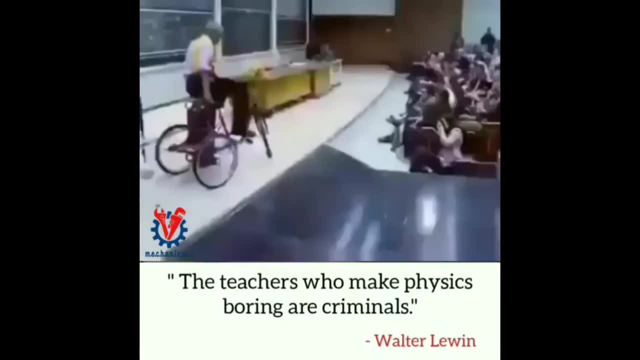 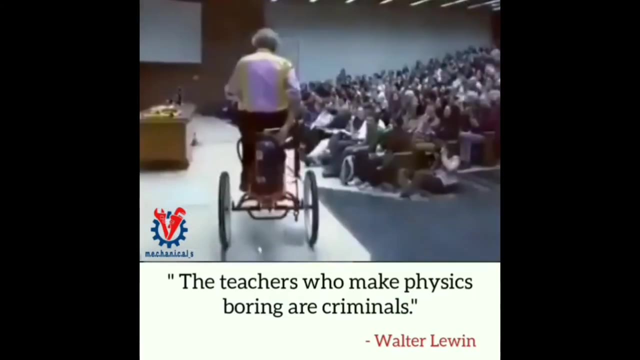 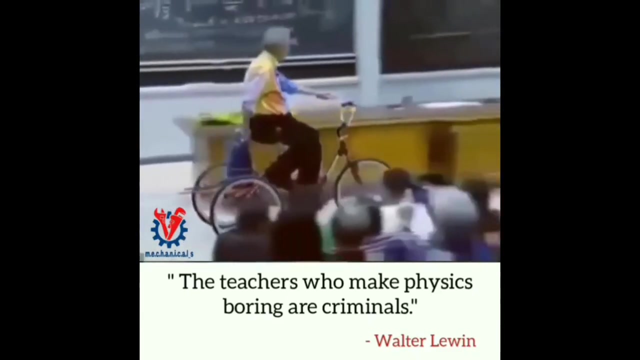 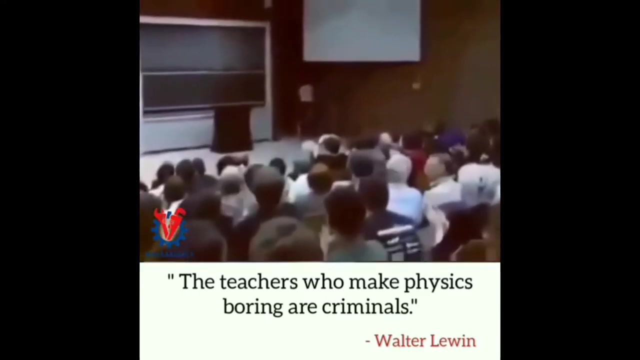 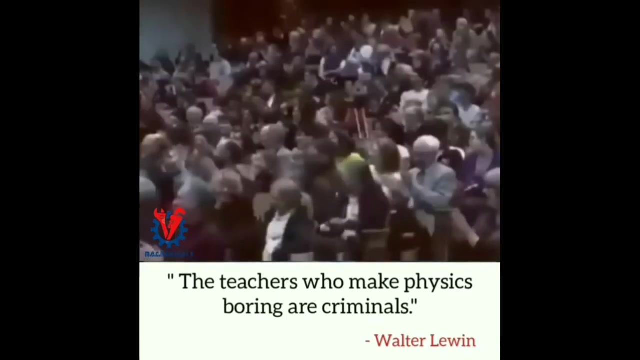 Yeah, Those of you who do not see blue say no, No, You better see an eye doctor, And then your eyes get darkened. An eye doctor means just one thing: You don't see the light. You don't see the light. 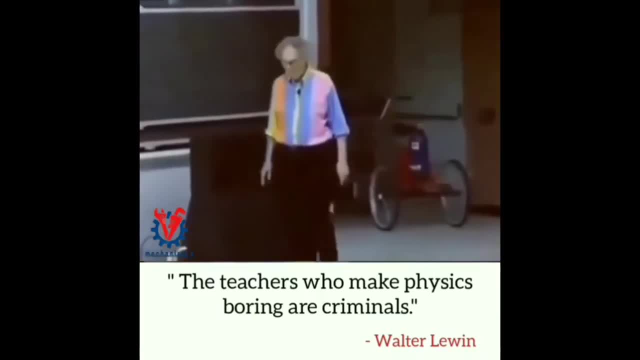 You look at yourself and say: I see the light, You see the light, And then you see the light, And that light comes back and you'll see the light again when you get down. But the light is not the troubles with which we are talking. 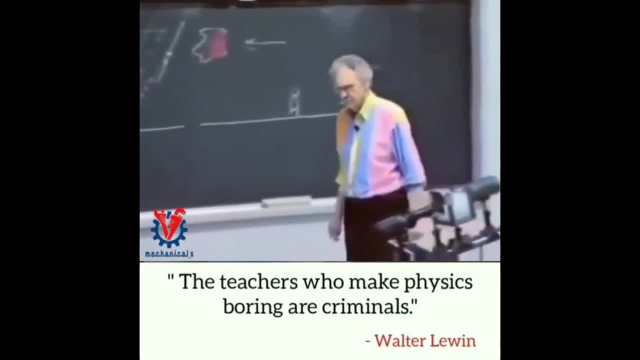 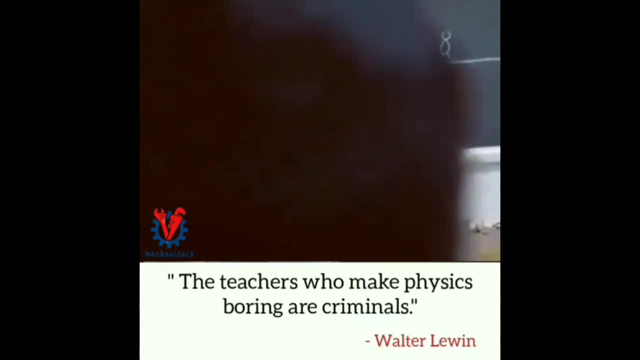 Oh, that's amazing. I could do it for my doctor. It's a miracle just about to happen. Yeah, I know, I'm glad, I'm glad, I'm glad Really. Yeah, I'm glad, It's a good day. 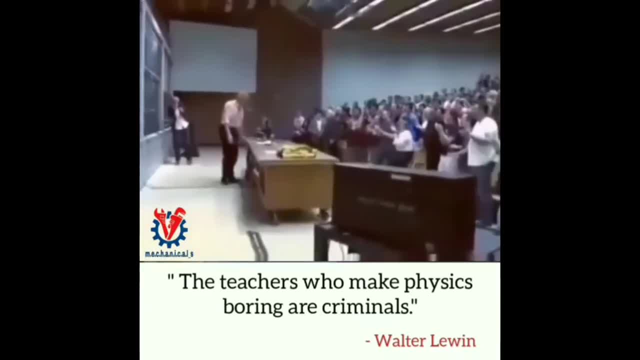 I'm happy, I'm happy, Thank you, I'm happy, Thank you, Thank you, Thank you.